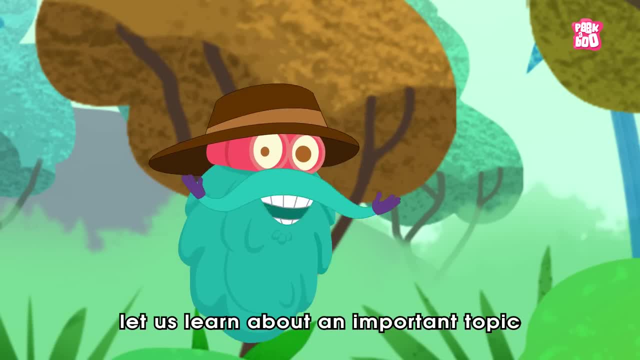 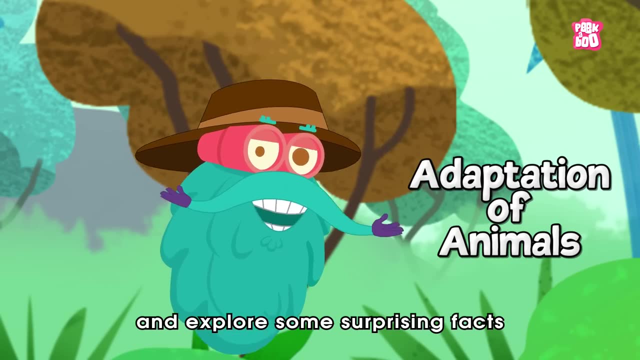 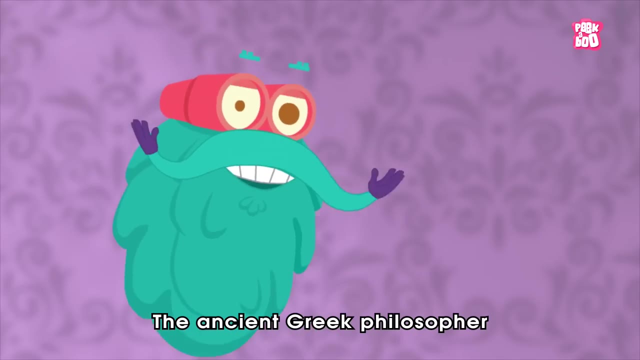 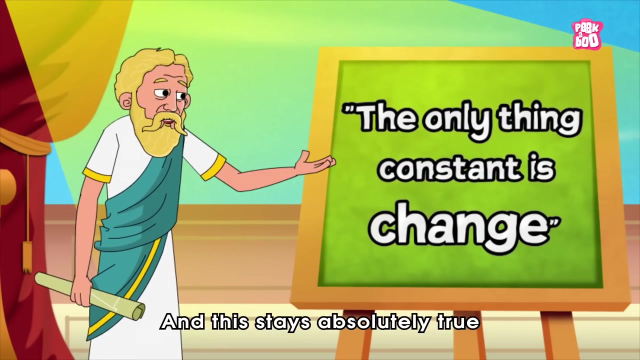 Hey friends, in today's episode, let us learn about an important topic called adaptation of animals and explore some surprising facts behind it. Zoom in. The ancient Greek philosopher Heraclitus once said: The only thing constant is change, And this stays absolutely true when it comes to the animal kingdom. 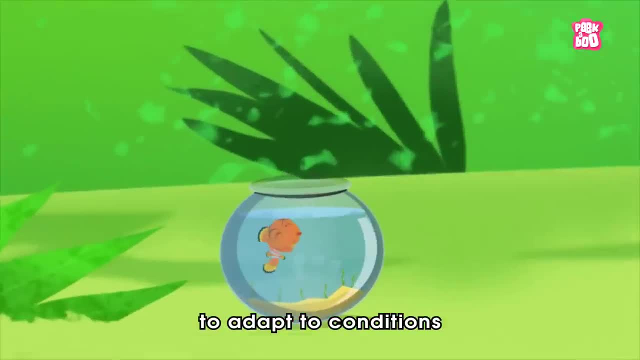 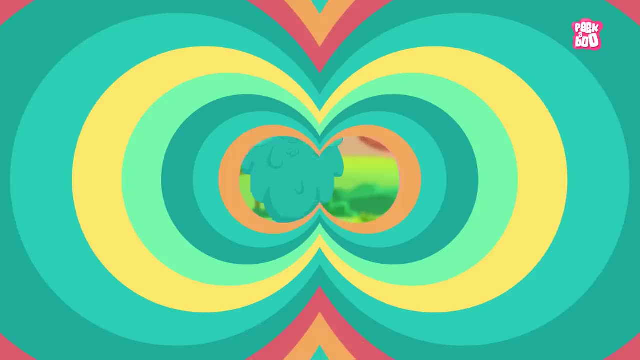 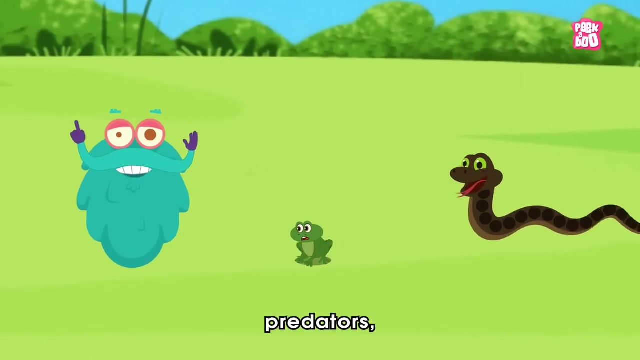 as they need to find ways to adapt to conditions that are gradually or suddenly different from pre-existing ones. This means adapting to survive the climatic conditions of the ecosystem, predators and other animals that compete for the top. It is even the same for the same food and resources. 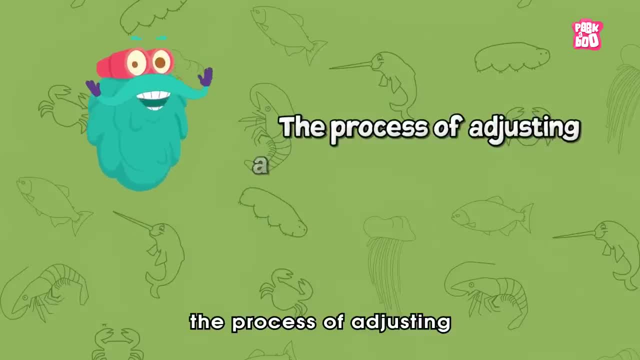 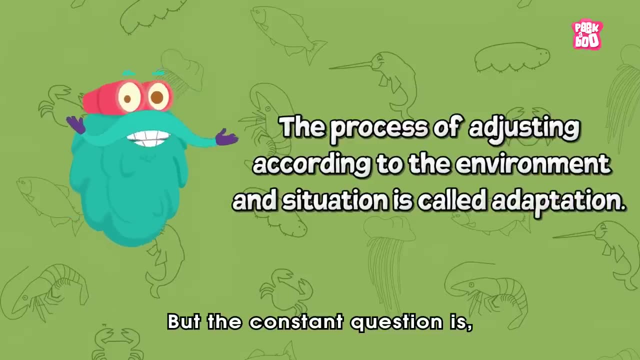 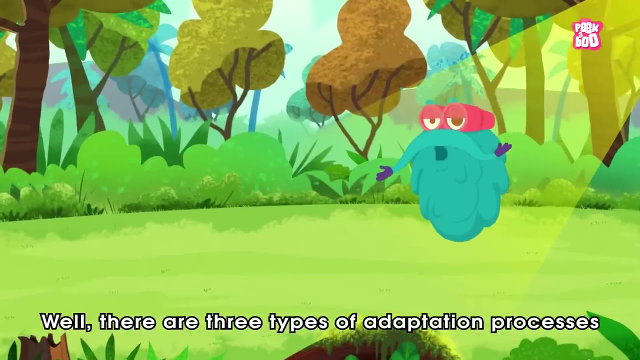 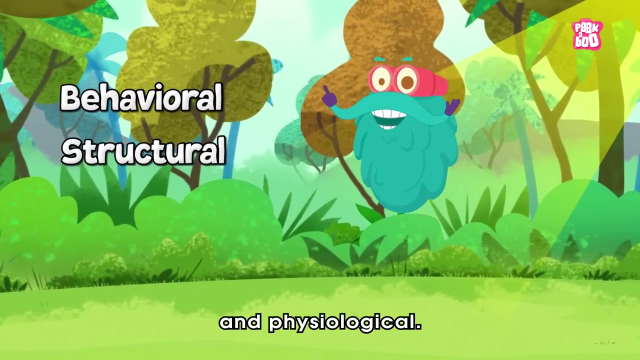 In simple words, the process of adjusting according to the environment and situation is called adaptation. But the constant question is: how do these animals adapt? Well, there are three types of adaptation processes in the animal world, that is, behavioral, structural and physiological. 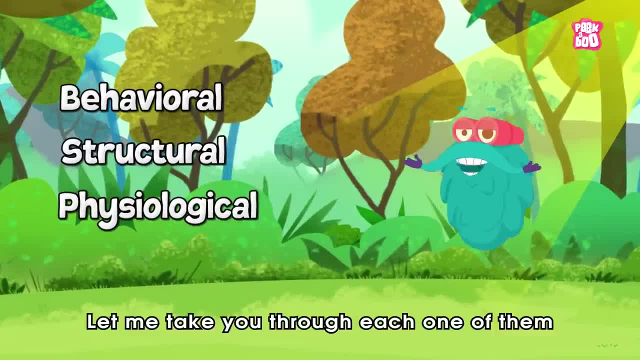 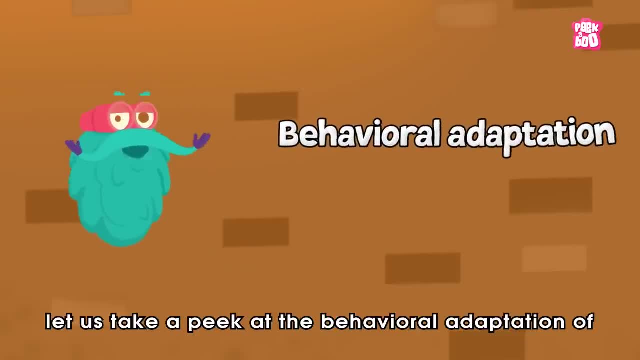 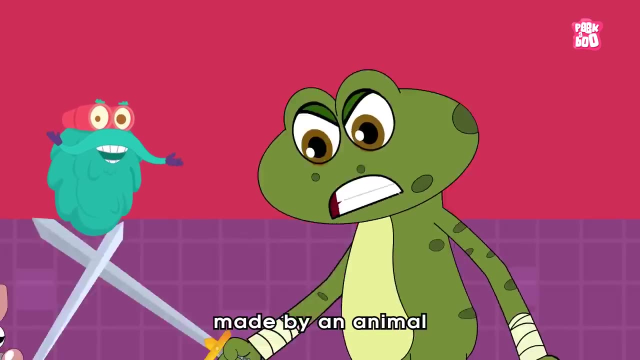 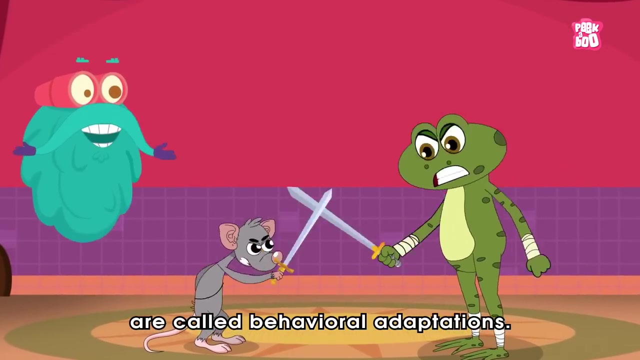 Let me take you through each one of them one by one. First, let us take a peek at the behavioral adaptation of animals. Adaptations that affect how an organism acts or responses made by an animal that helps it to survive and reproduce are called behavioral adaptations. 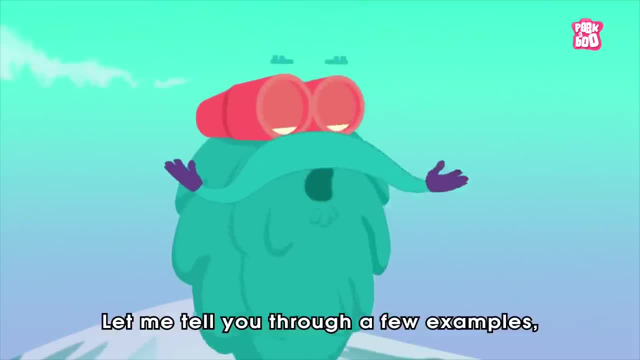 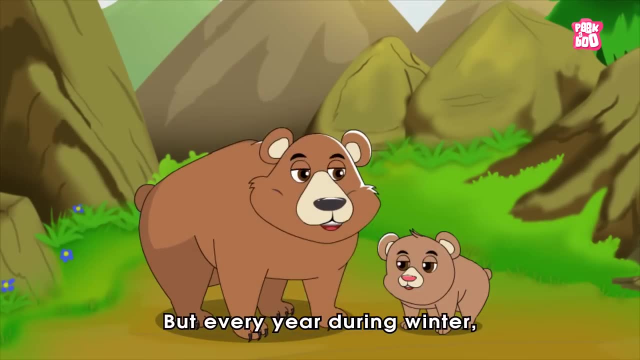 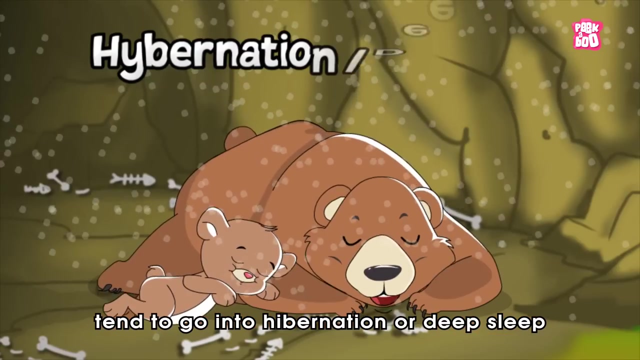 Let me tell you through a few examples. As we know, bears are very active and energetic animals, But every year, during winter, some of the bear species tend to go into hibernation or deep sleep, depending upon the snowfall, temperature and food supply. 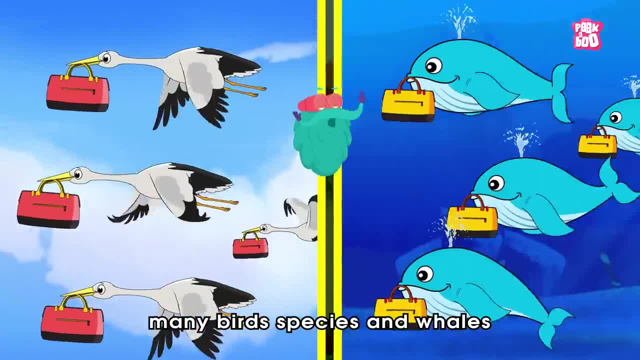 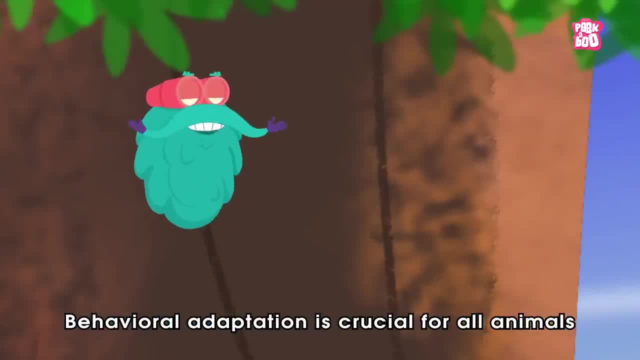 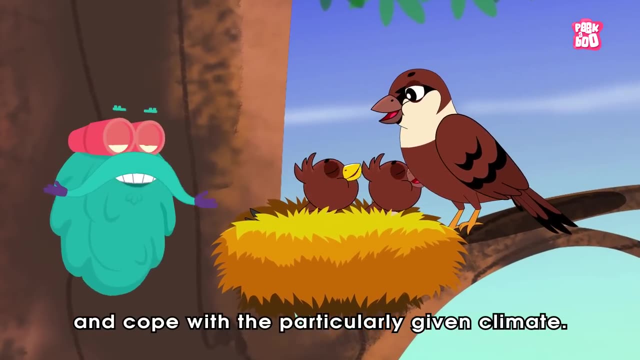 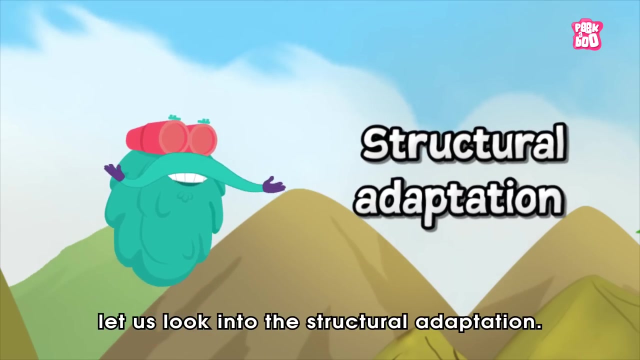 Similarly, many bird species and whales tend to migrate to a warm environment. Behavioral adaptation is crucial for all animals to find ways to raise the food they need and cope with the particularly given climate. Next, let us look into the structural adaptation. and what is that? 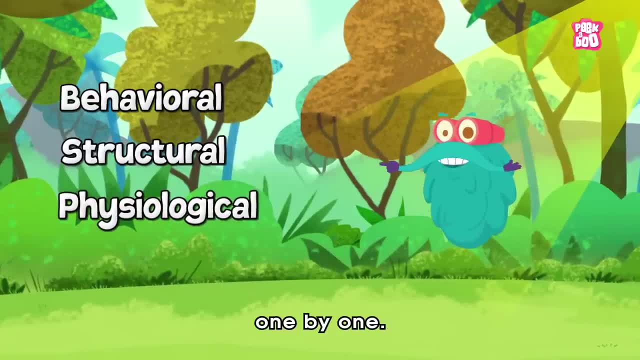 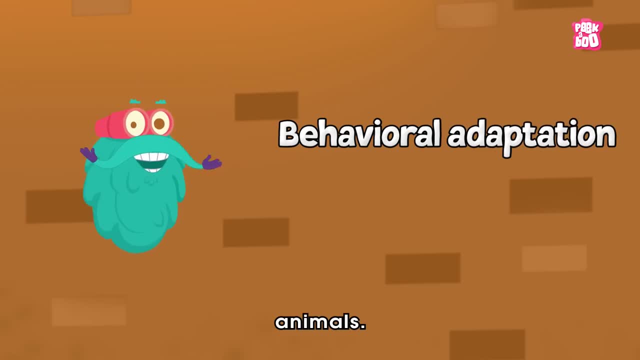 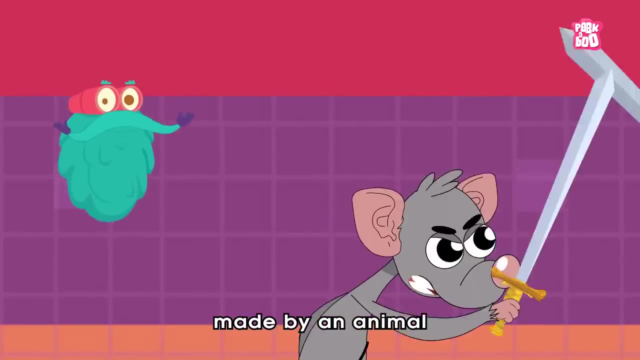 Let me take you through them. Let me take you through each one of them one by one. First, let us take a peek at the behavioral adaptation of animals. Adaptations that affect how an organism acts or responses made by an animal that helps it to survive and reproduce are called behavioral adaptations. 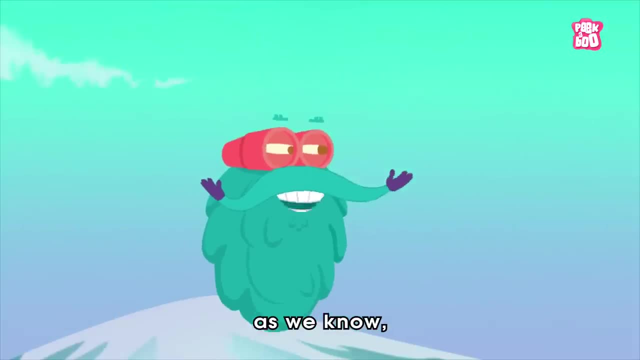 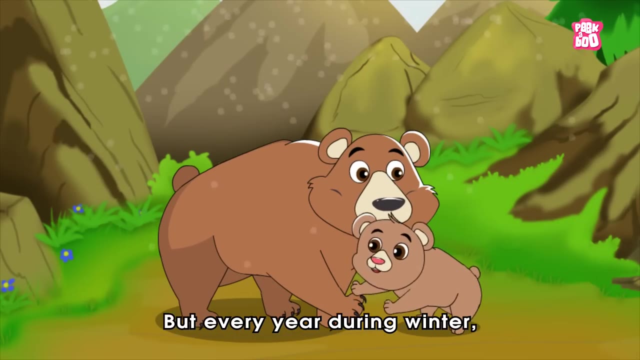 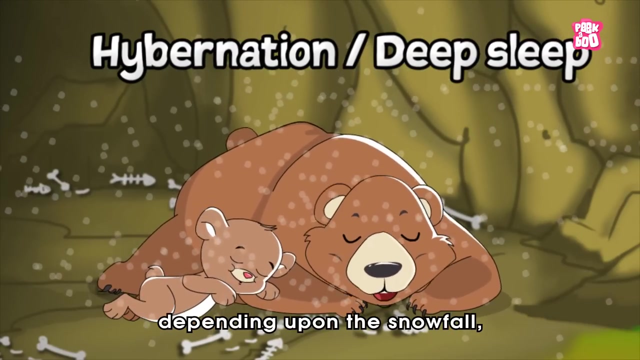 Let me tell you through a few examples. As we know, As we know, As we know, Behavioral adaptations are very active and energetic animals, But every year, during winter, some of the best species tend to go into hibernation or deep sleep, depending upon the snowfall, temperature and food supply. 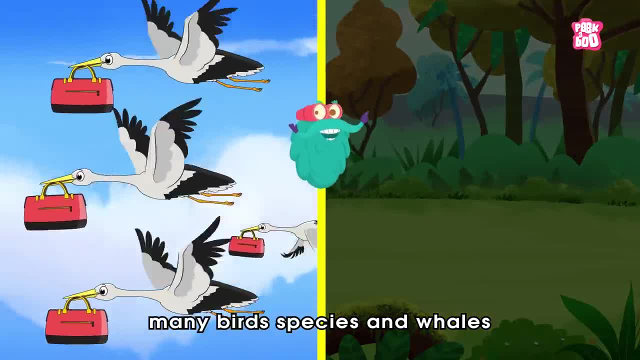 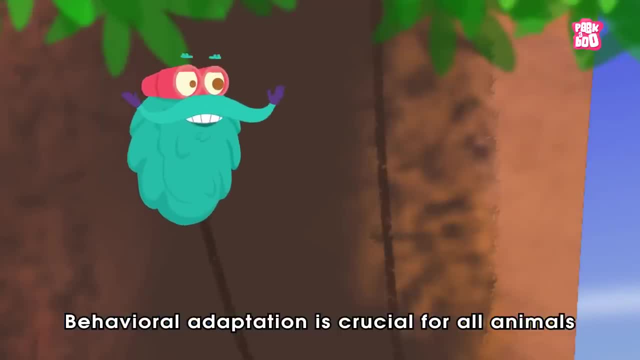 Similarly, many bird species and whales tend to migrate to a warmer place during winter. Behavioral adaptation is crucial for all animals. Behavioral adaptation is crucial for all animals. If you are really smart enough to learn how to adapt to an organism, try postponing a disciplinary. जा उतोदारिंहण नहरा ख किपाल master. 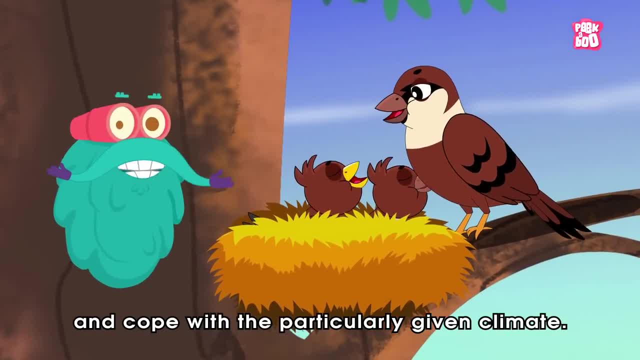 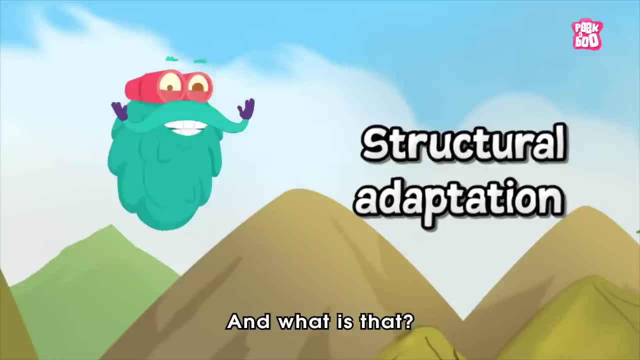 you will learn how a bee can lift a worry-side insect- you don't even want the bee to fall onwards- and how to save crimes on earth if the bee is too violent in nature. Next, let us look into the structural adaptation and what it is that. 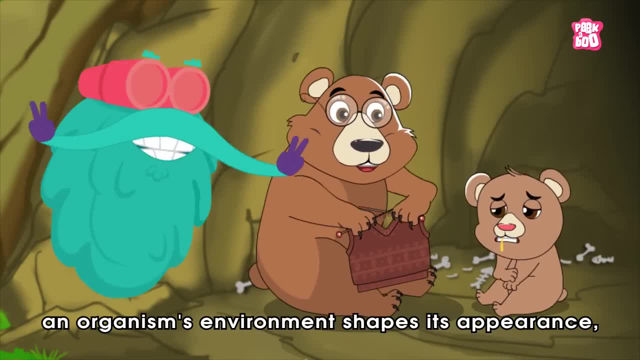 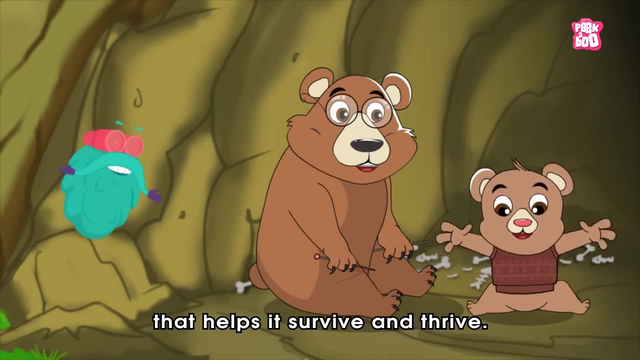 In this process, an organism's environment shapes its appearance. meaning an organism develops a body feature that helps it survive and thrive. meaning an organism develops a body feature that helps it survive and thrive. It may be in the way the body works in certain elements of the body. 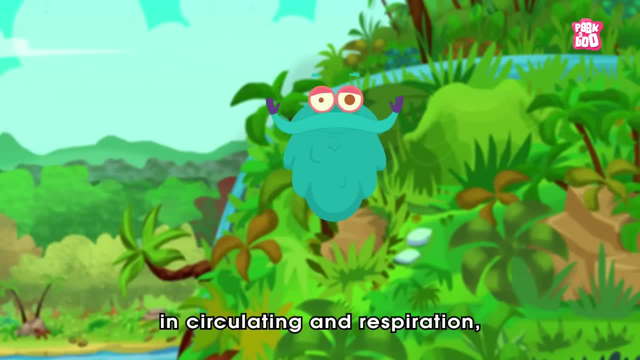 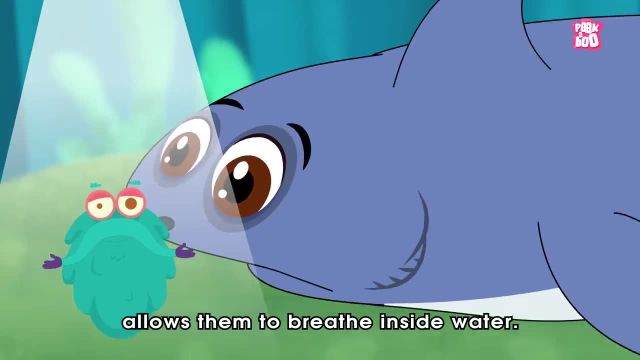 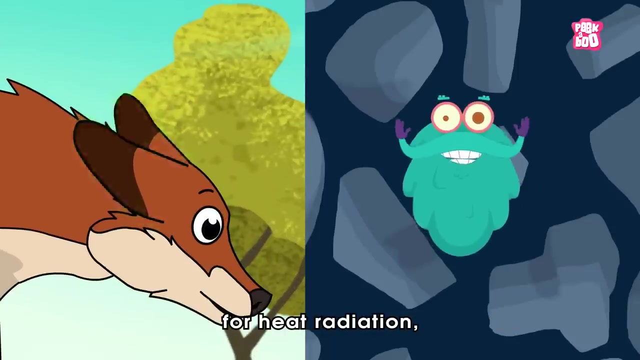 It may be in the way the body works in certain elements of the body, in circulating and respiration, for instance, the gills that fishes have allows them to breathe inside water. or, as you must have noticed, that the desert foxes have large years for heat radiation. 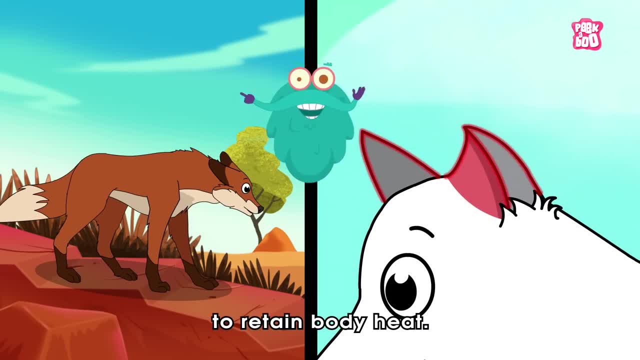 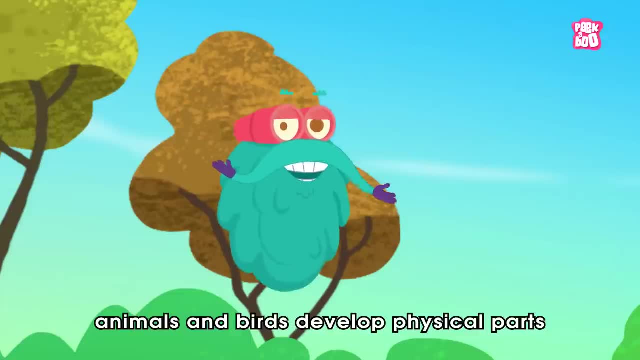 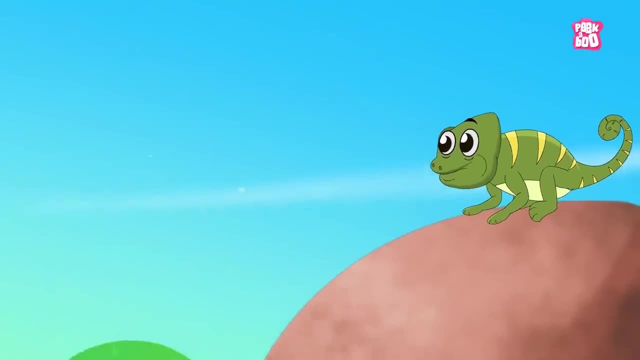 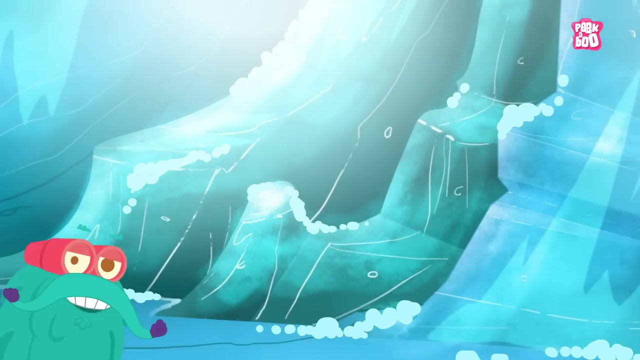 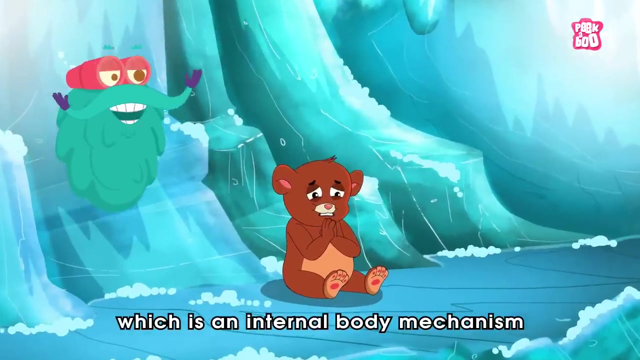 the arctic foxes have small years to retain body heat. in short, in structural adaptation, animals and birds develop physical parts through evolution that allow them to find and consume food, defend themselves and reproduce their species. and last comes the physiological adaptation, which is an internal body mechanism of an animal. 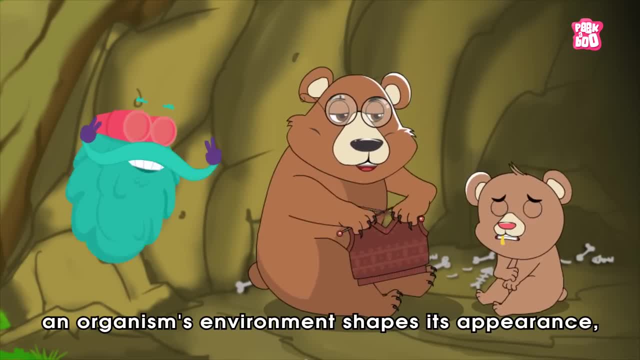 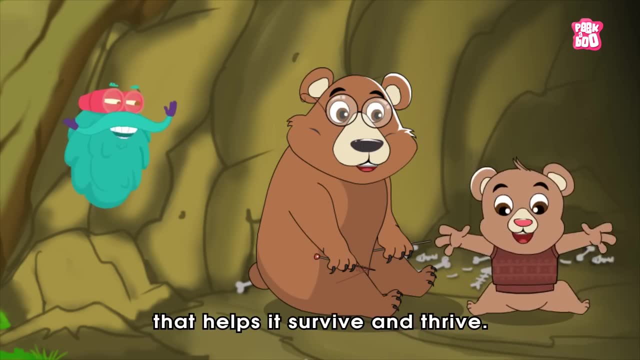 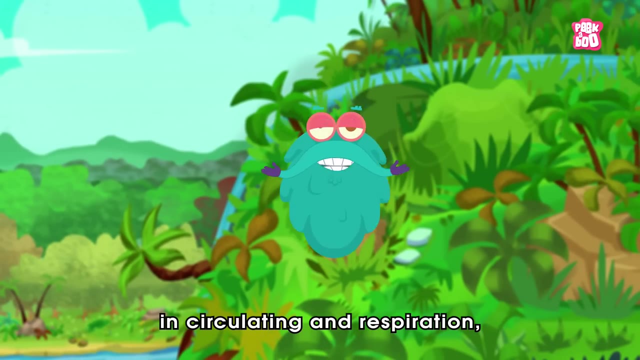 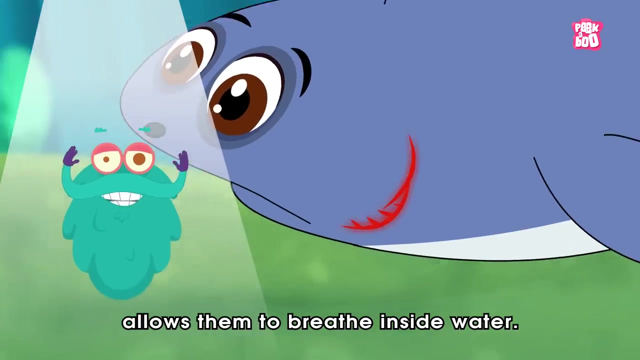 In this process, an organism's environment shapes its appearance, Meaning an organism develops a body figure, A creature that helps it survive and thrive. It may be in the way the body works, in circulating and respiration. For instance, the gills that fishes have allows them to breathe inside water. 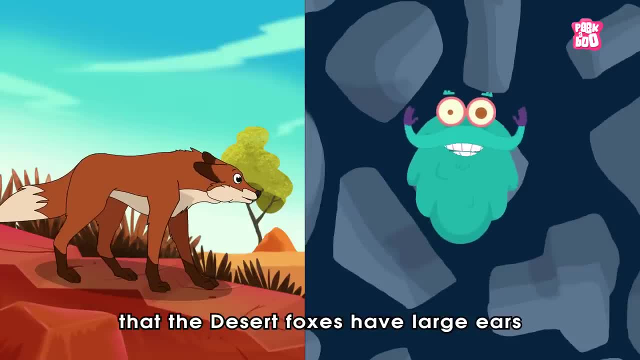 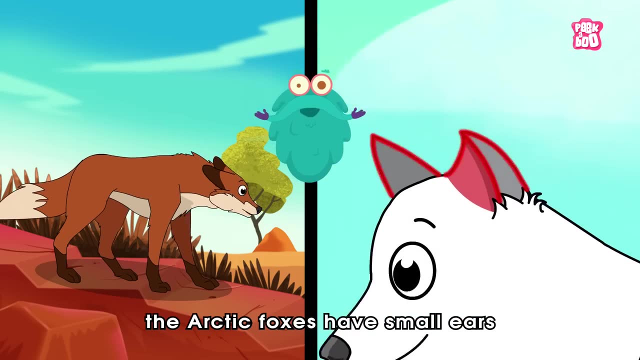 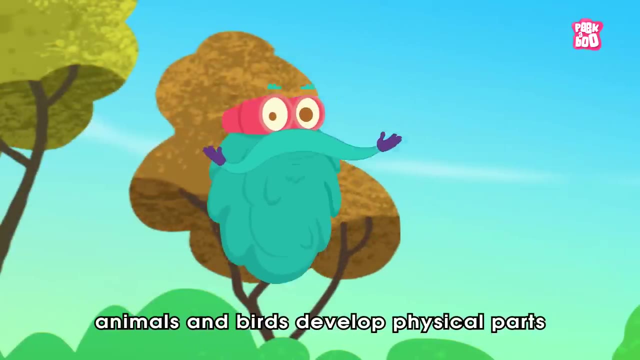 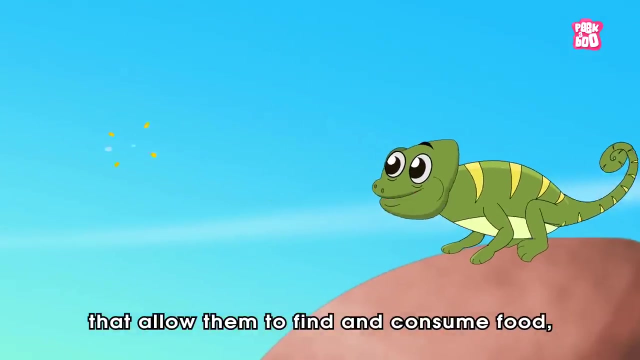 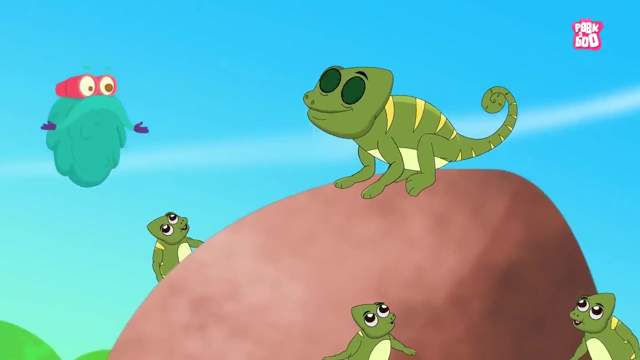 Or, as you must have noticed, that the desert foxes have large ears for heat radiation, The arctic foxes have small ears to retain body heat. In short, in structural adaptation, animals and birds develop physical parts through evolution that allow them to find and consume food, defend themselves and reproduce their species. 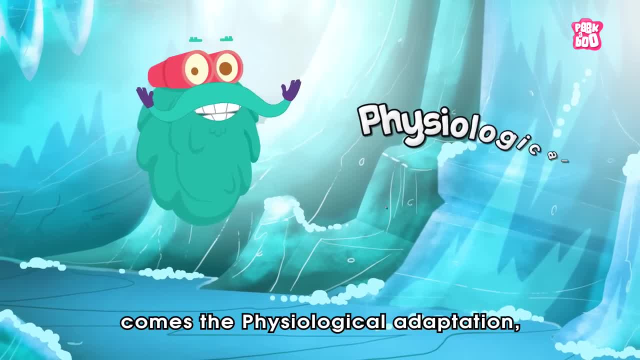 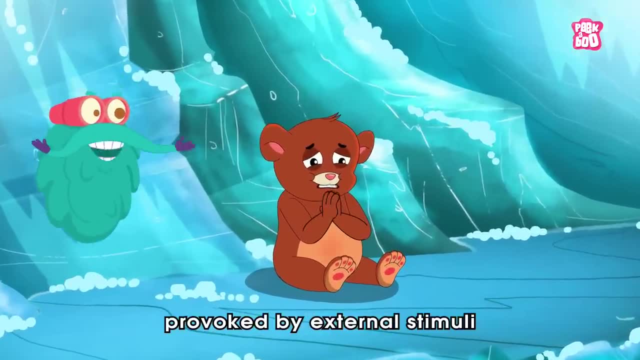 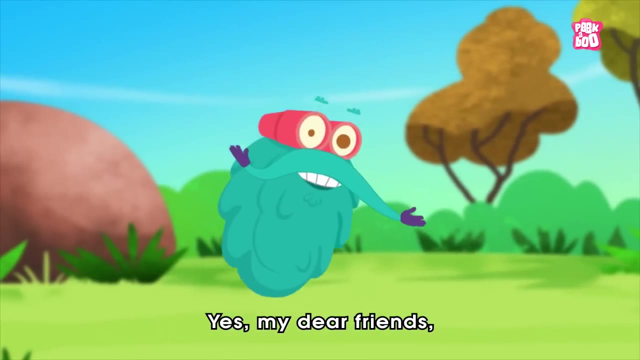 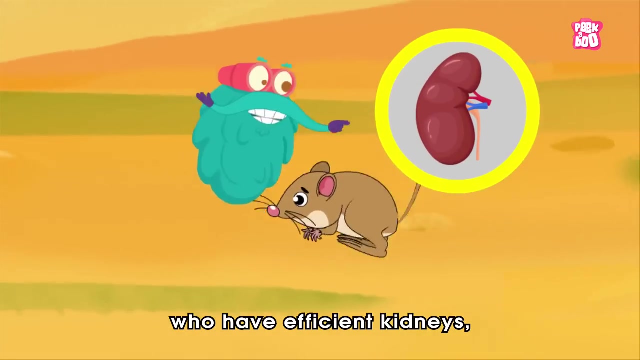 And last comes the physiological adaptation, Which is an internal body mechanism of an animal provoked by external stimuli That helps them to survive and reproduce. Yes, my dear friends, things like metabolism and body chemistry play a crucial role during this process. We can notice this phenomenon in animals like kangaroo rats, who have efficient kidneys. 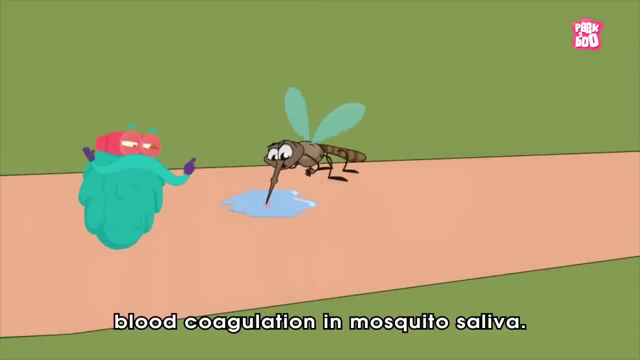 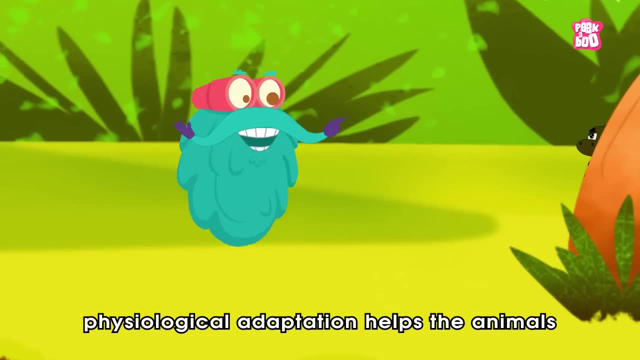 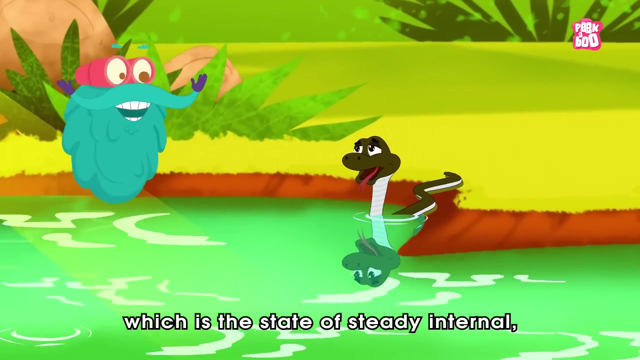 Or the presence of compounds that prevent blood coagulation in mosquito saliva. In other words, physiological adaptation helps the animals to maintain body equilibrium, or homeostasis, Which is the state of steady internal physical and chemical conditions maintained by living systems. 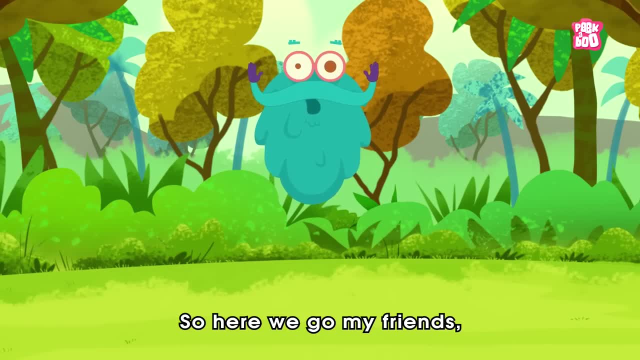 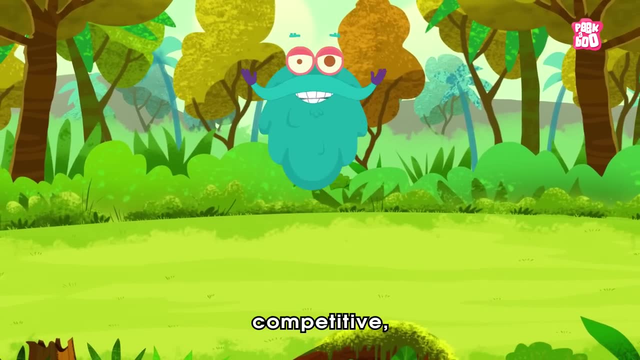 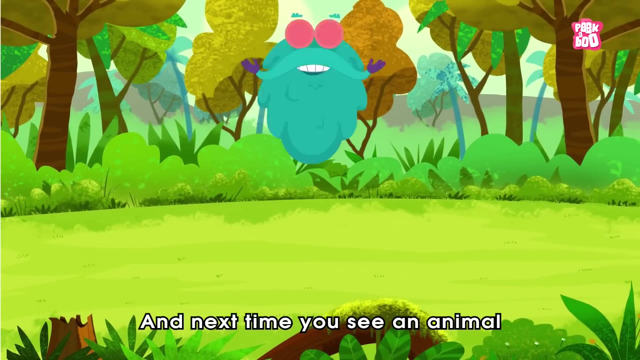 So here we go, my friends. Now you know how these wonderful animals manage to survive in a challenging, competitive and ever-changing environment With the help of adaptation. And next time you see an animal behaving and acting in a certain way. 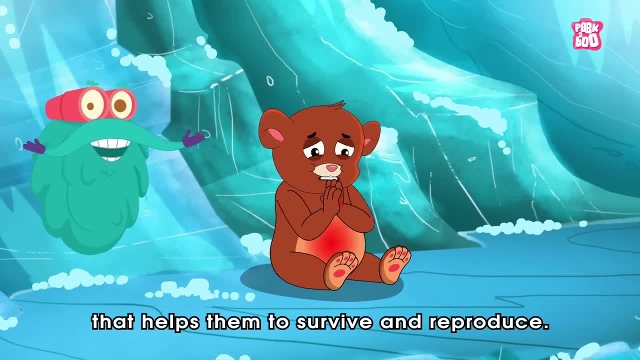 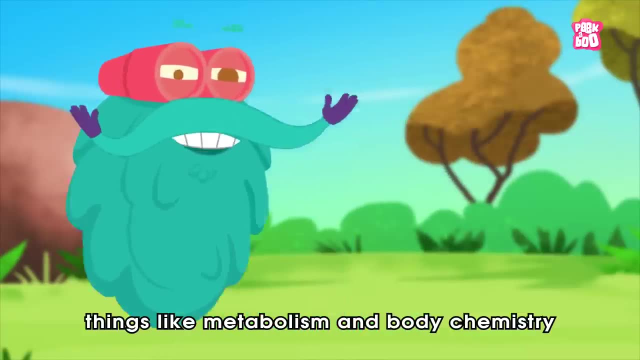 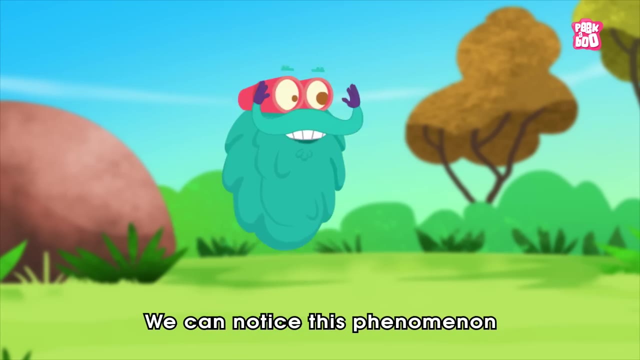 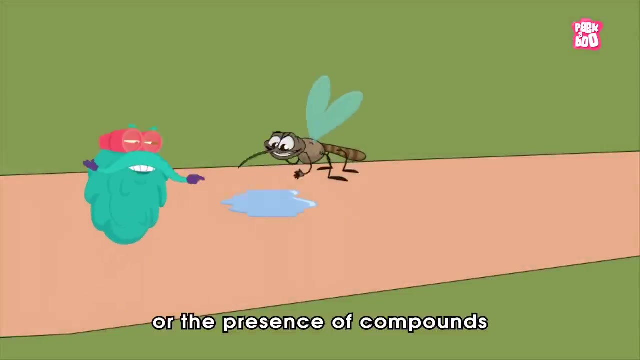 provoked by external stimuli that helps them to survive and reproduce. yes, my dear friends, things like metabolism and body chemistry play a crucial role during this process. we can notice this phenomenon in animals like kangaroo rats, who have efficient kidneys, or the presence of compounds that prevent blood coagulation in mosquito saliva. 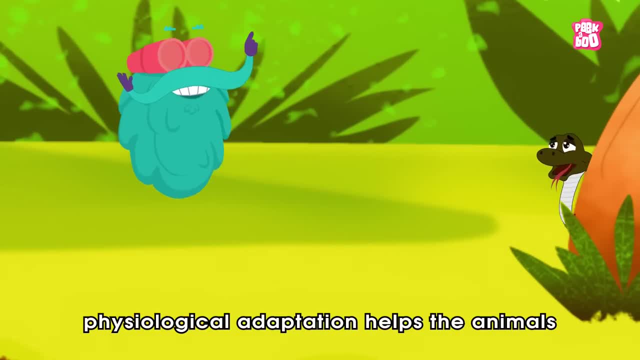 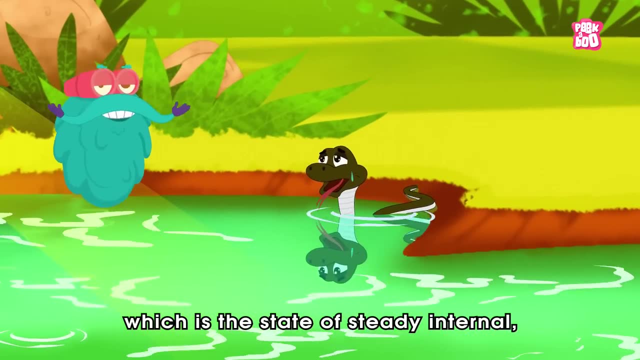 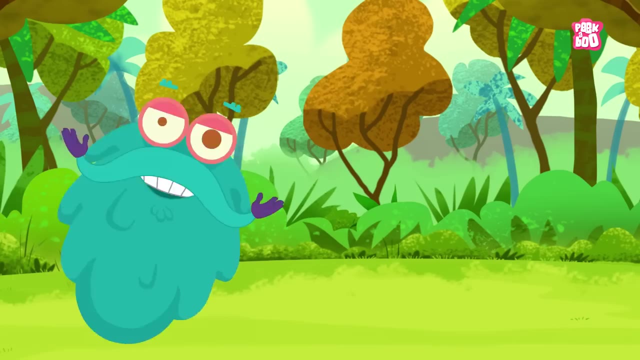 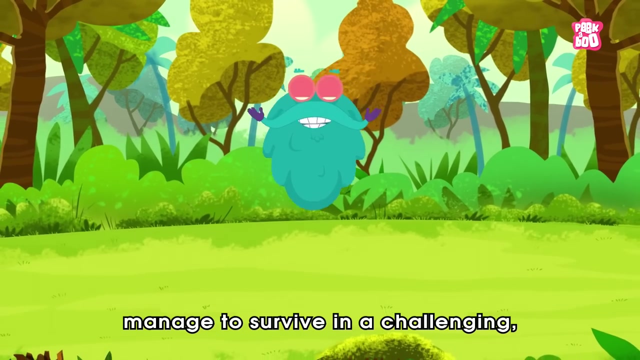 in other words, physiological adaptation helps the animals to maintain blood and body equilibrium, or homeostasis, which is the state of steady internal physical and chemical conditions maintained by living systems. so here we go, my friends. now you know how these wonderful animals manage to survive in a challenging, competitive and ever-changing environment. 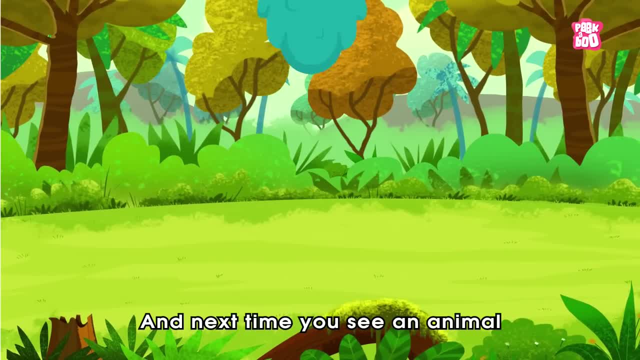 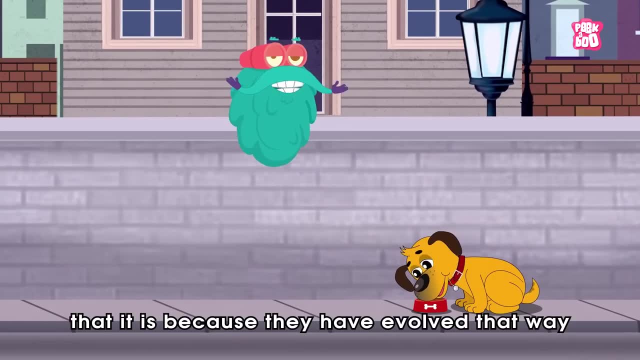 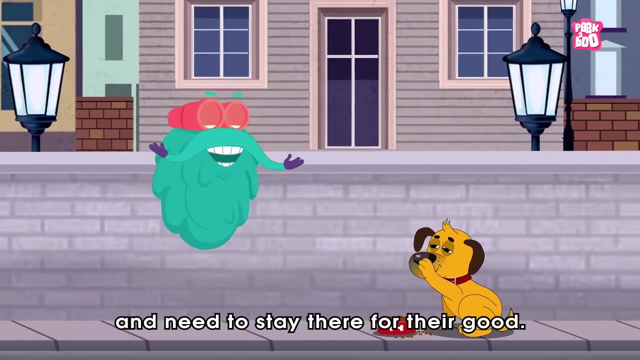 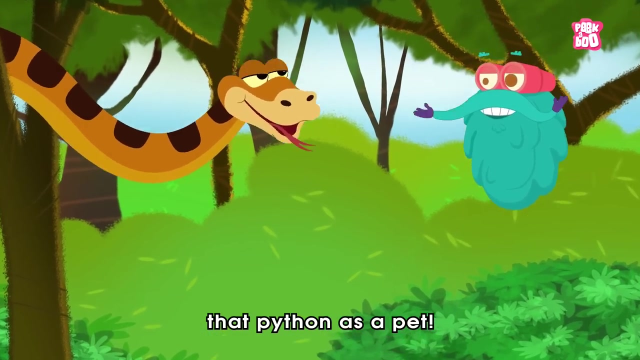 with the help of adaptation, and next time you see an animal, you will know that it is the animal that has the most potential to survive and act in a certain way. always remember that it is because they have evolved that way, according to their ecosystem, and need to stay there for their good. no wonder your parents refuse to. 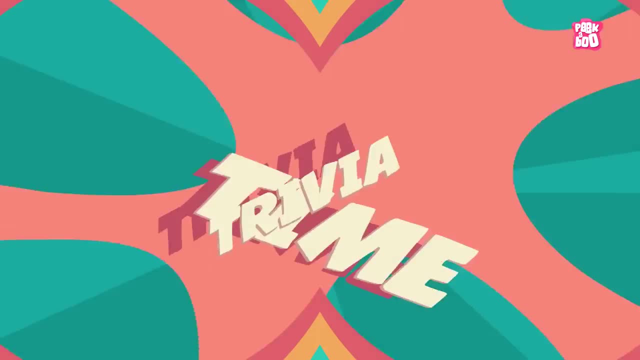 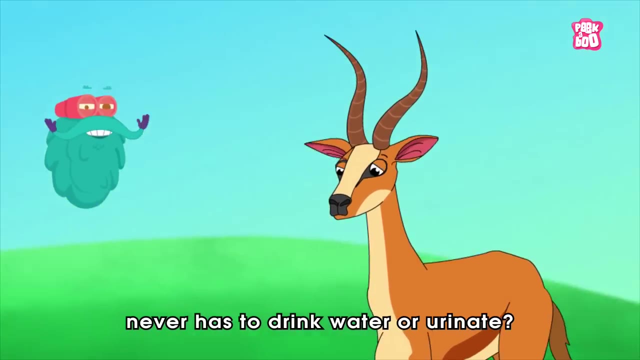 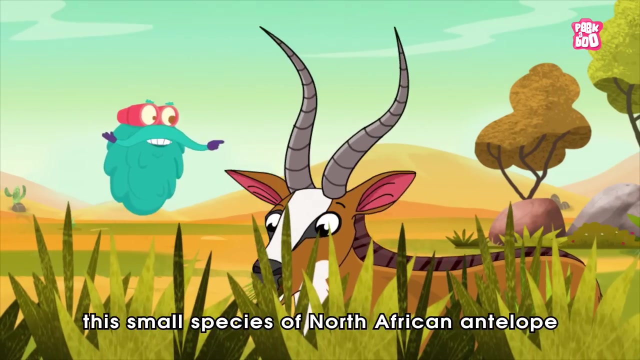 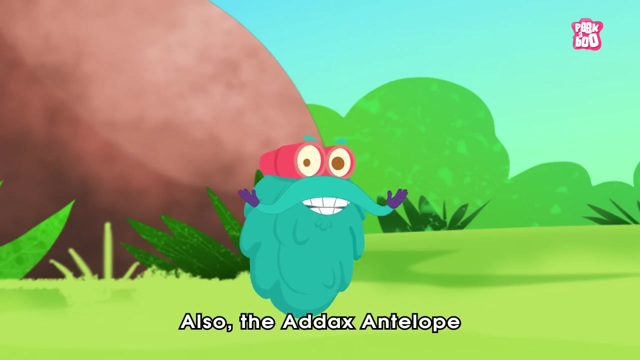 adopt that python as a pet trivia time. did you know? the darkest gazelle never has to drink water or urinate. yes, though, they will drink water when it's available. this small species of north african antelope can get all the water it needs from the food in its diet. also the adax antelope. 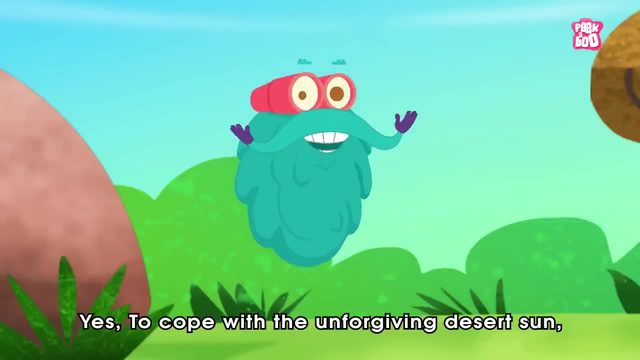 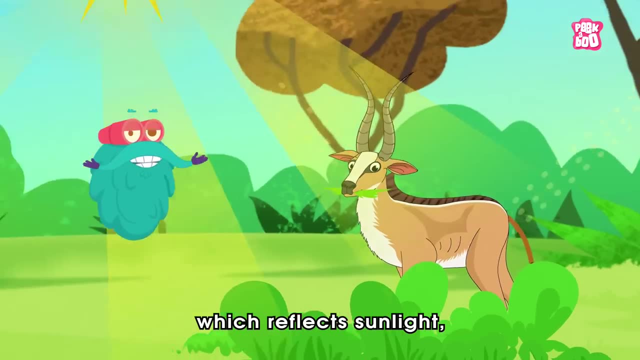 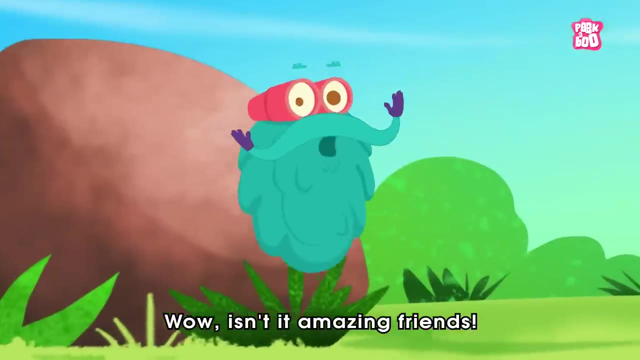 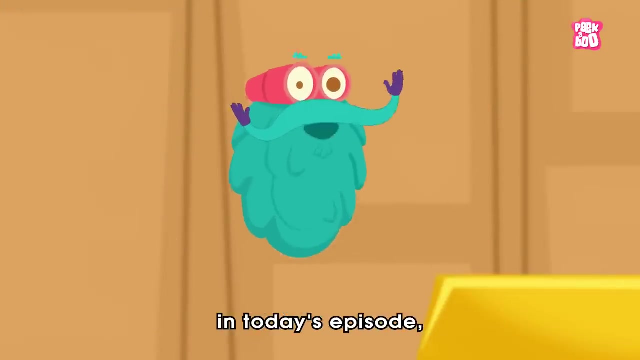 changes color with the seasons. yes, to cope with the unforgiving desert sun, the adax sports a white coat in the summer, which reflects sunlight, but in winter the coat turns brownish gray to better absorb heat. wow, isn't it amazing, friends, hope you learned something new in today's episode. until next time, it's me dr bynox, zooming out. ah, never mind.